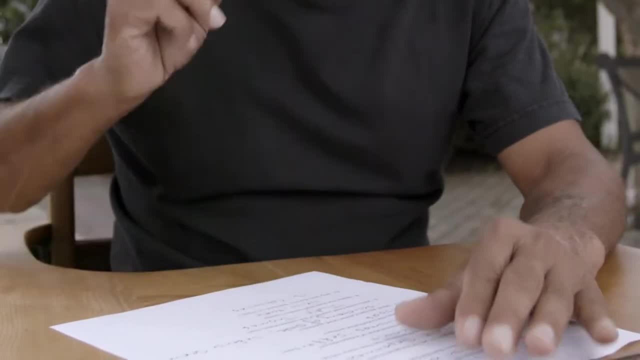 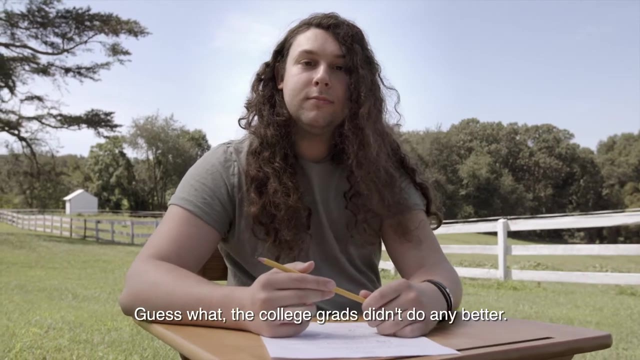 I'm going to guess 24.. But I don't. I know this stuff because I had to study it to become a US citizen. I'm a high school graduate. I don't think I did that well. Guess what The college you've credits to you do any better. 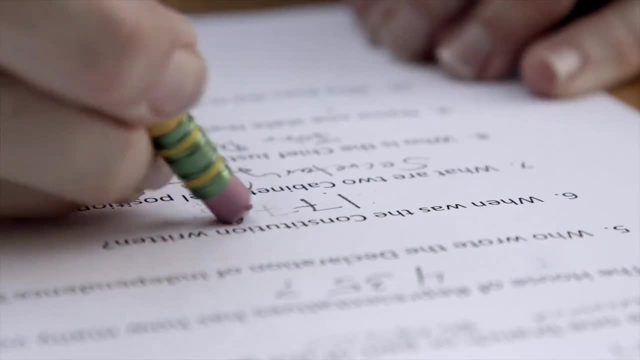 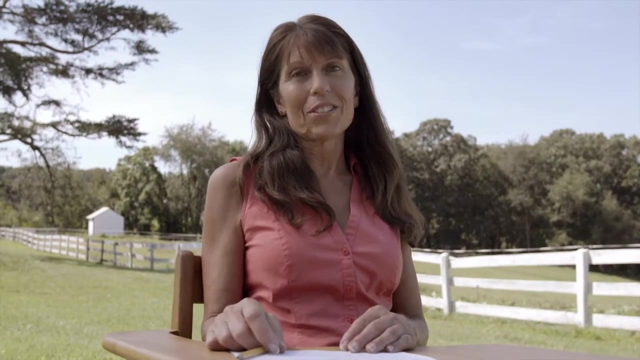 I have a master's degree in strategic communications and I think I utterly failed this test. I am an educated person and I'm an educator also, so I probably should know this much better than I do. Hey, I can serve myself. 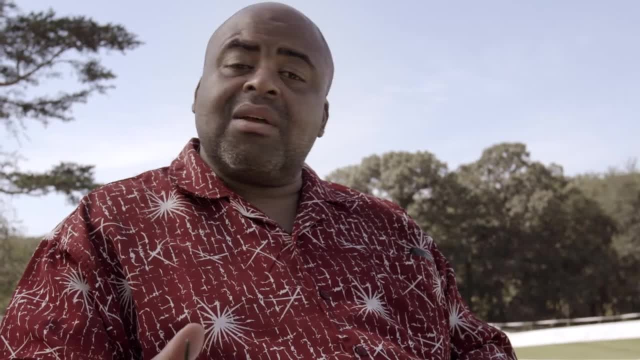 I'm pretty knowledgeable and informed. No, I really didn't know it at all, though I should definitely know more about the way our government is run. You know, I kind of think that knowledge is power, so I think the more that people would know this stuff, the better it would benefit society. You know, I kind of think that knowledge is power. so I think the more that people would know this stuff, the better it would benefit society. 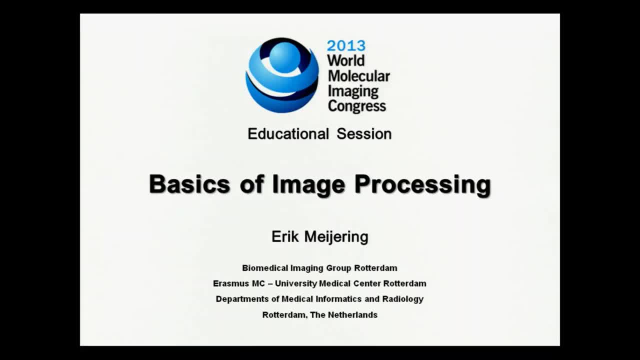 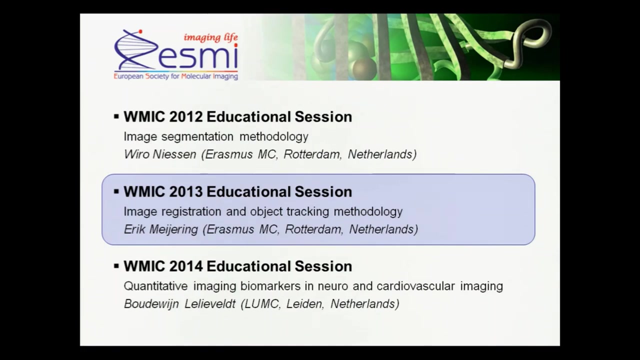 Welcome to this educational session on the basics of image processing, and I will be talking to you about image registration and tracking in particular. So just to sketch the context. so this is a lecture in a series of three. Last year, Vero Niessen from the Erasmus Medical 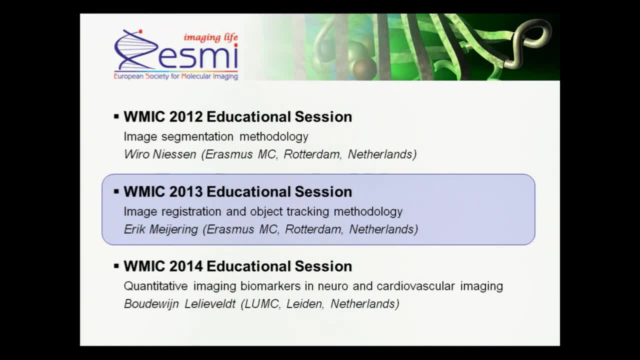 Center in Rotterdam. he spoke about methods for image segmentation. So how to using a computer to automatically recognize objects in the images and to outline them? And this year I will be talking about image registration and object tracking, as I told you. And next, 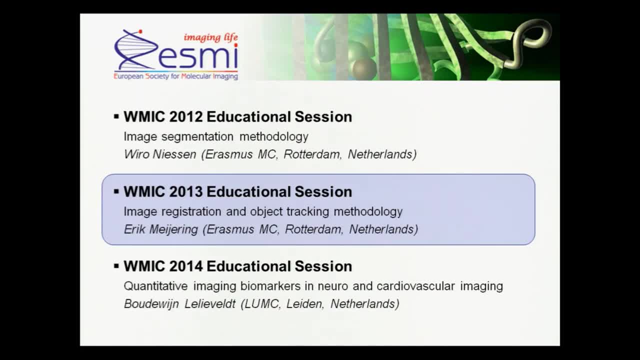 year there will be a session by Boudewijn Lelyveld from Leiden University Medical Center, And he will be talking about quantitative imaging biomarkers, in particular in neuro and cardiovascular imaging. And before I forget, I would like to first acknowledge 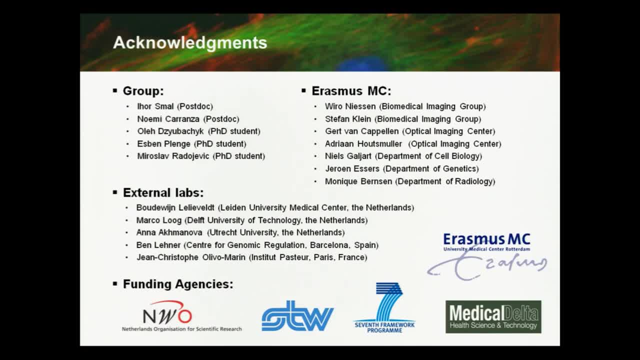 a bunch of people: the postdocs and PhD students in my own group, but also other people at Erasmus Medical Center. Vero Niessen I already mentioned. Stefan Klein is also in our group and does a lot of work on image registration. I used some of his slides And also the external.